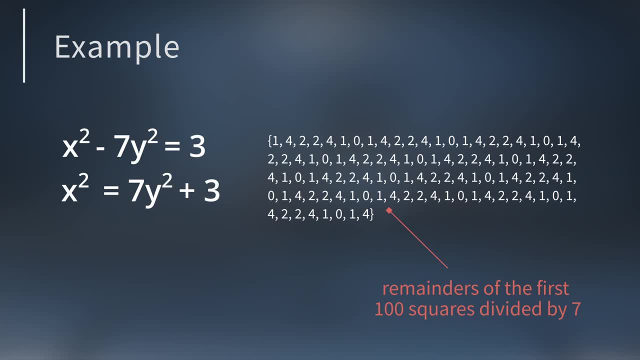 squares when you divide by 7.. There is a clear pattern: If you divide the square of an integer by 7, then you get zero, one, two or four. While we won't show it here, this pattern is a little bit different. If you divide the square of an integer by 7, then you get 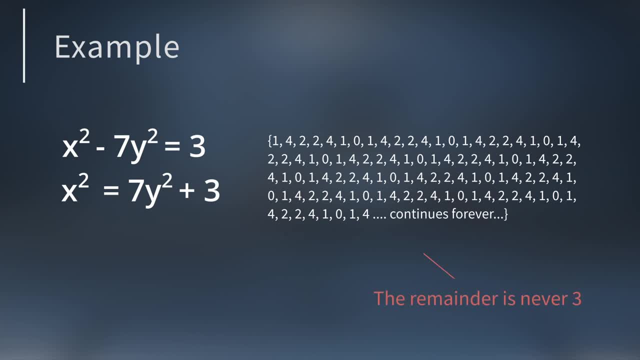 zero, one, two or four, While we won't show it here- this pattern is a little bit different- does continue forever. that's important, but you never get a remainder of 3, so there are no solutions to the Diophantine equation, The key to this. 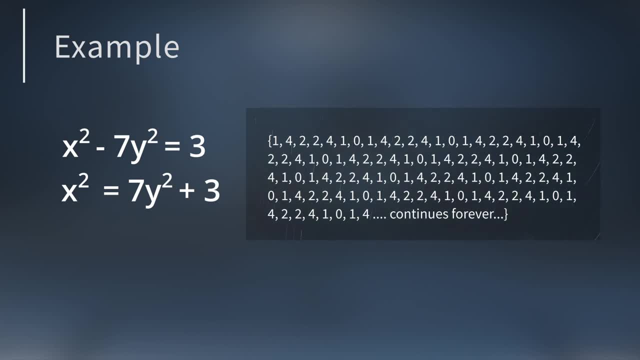 solution was to observe a pattern in the remainders of squares when you divide by 7. Namely, there are only four possible remainders, but if you look more closely you'll see the remainders repeat in a block of 7.. Now to be responsible. 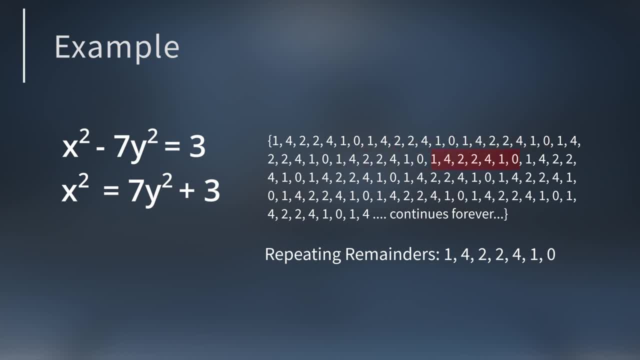 mathematicians. we'd still want to show that this pattern does hold, but for now, it's enough to see the pattern. This is an example of how working with remainders enables you to solve what appears to be a challenging problem. Let's use this as 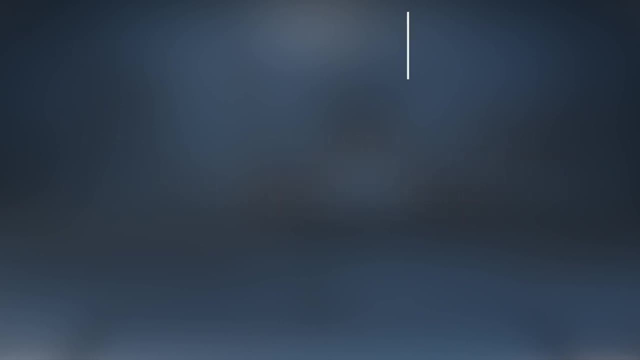 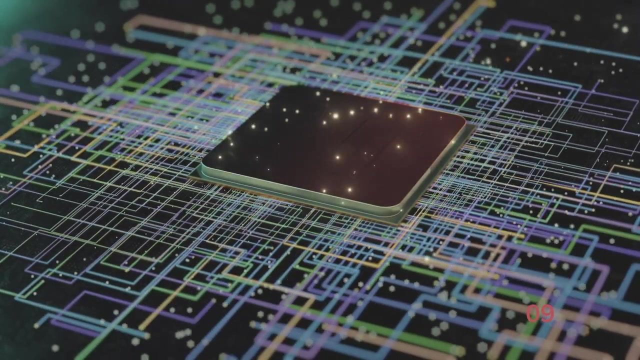 a springboard into the world of congruences. Because you're watching this video, we think you might enjoy math, science and programming, and that means you should check out our website, Socraticacom. We have courses- merch. 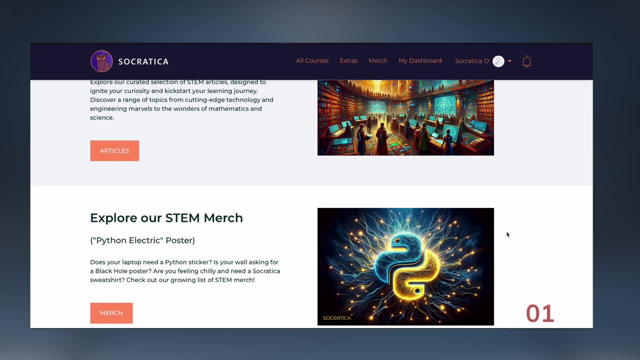 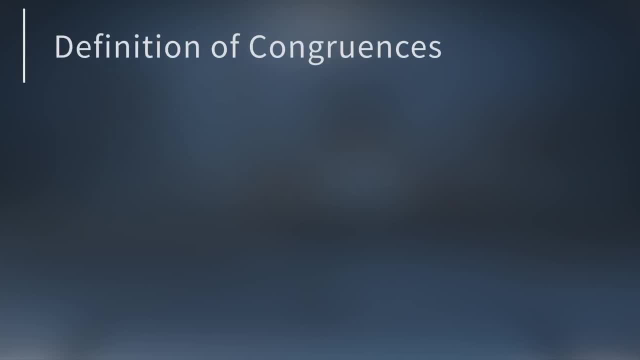 handouts, articles and more. There's so much to learn, and we'll help you learn more, Thank you. Thank you. Now on with the show. To define congruences, let's explore divisibility by seven in more detail. Here are a bunch. 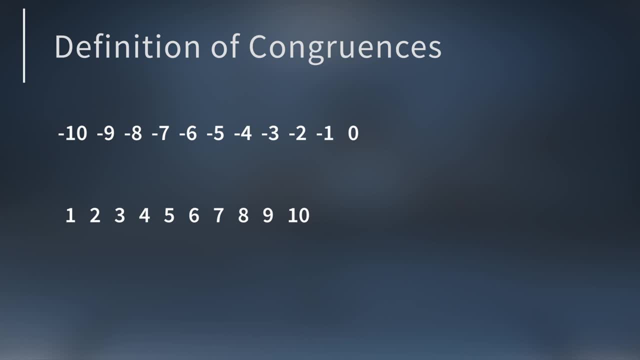 of integers, both positive and negative. If you divide each integer by seven, you get a remainder between 0 and 6.. Even when you divide a negative number by seven, you still get a remainder between 0 and 6.. Let's group the integers into sets by their remainder. 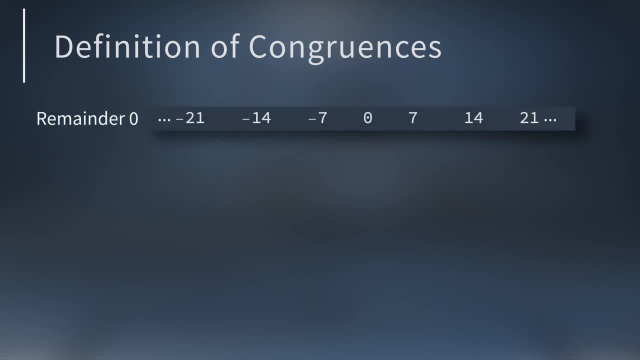 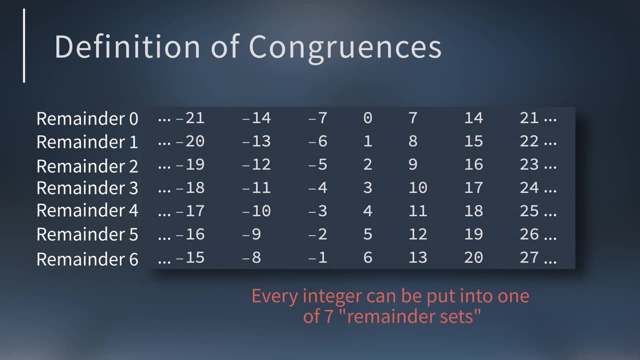 The first will be all the integers with a remainder of zero when you divide by seven. The next will be those with a remainder of one, then two and so on. So every integer can be put into one of seven remainder sets. In each set the integers are seven apart. 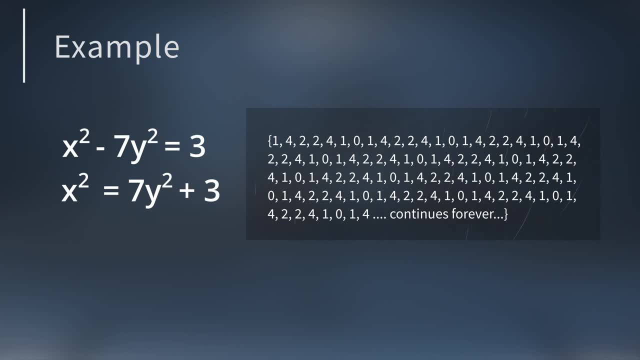 7. Namely, there are only four possible remainders, but if you look more closely, you'll see the remainders repeat in a block of 7.. Now to be responsible mathematicians. we'd still want to show that this pattern does hold, but for now, 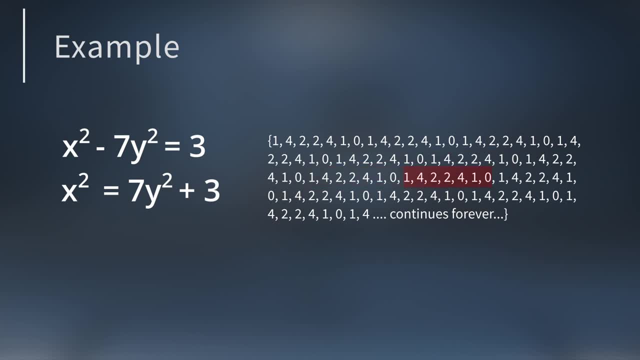 it's enough to see the pattern. This is an example of how working with remainders enables you to solve what appears to be a challenging problem. Let's use this as a springboard into the world of congruences, Because you're watching this. 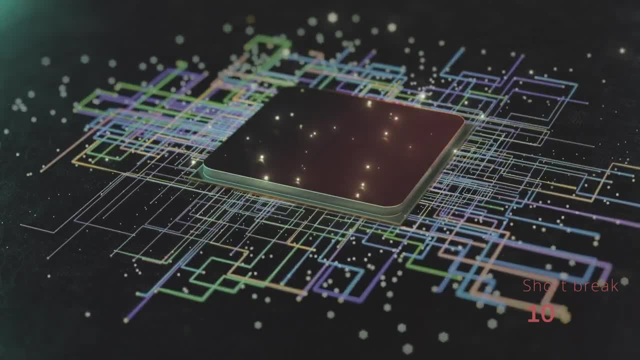 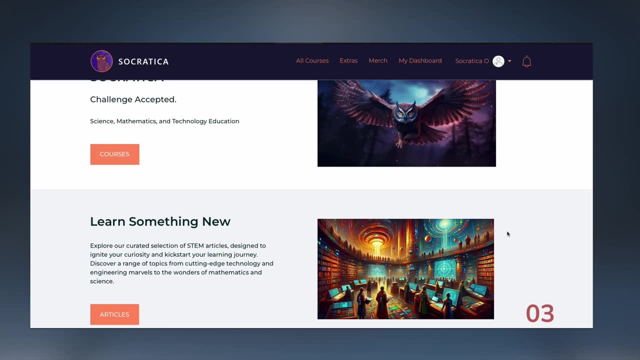 video. we think you might enjoy math, science and programming, and that means you should check out our website, Socraticacom. We have courses, merch handouts, articles and more. There's so much to learn and we'll help you learn. 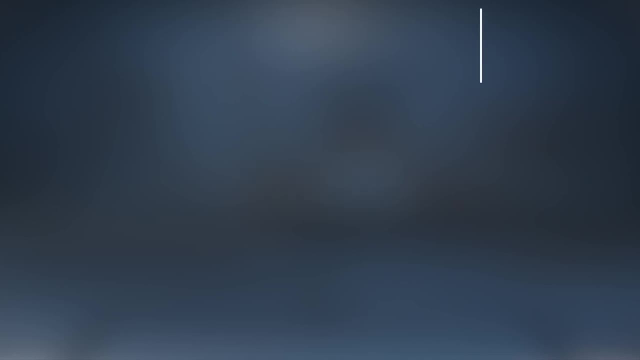 more, Thank you. Thank you. Now on with the show To define congruences. let's explore divisibility by seven in more detail. Here are a bunch of integers, both positive and negative. If you divide each integer by seven, you get: 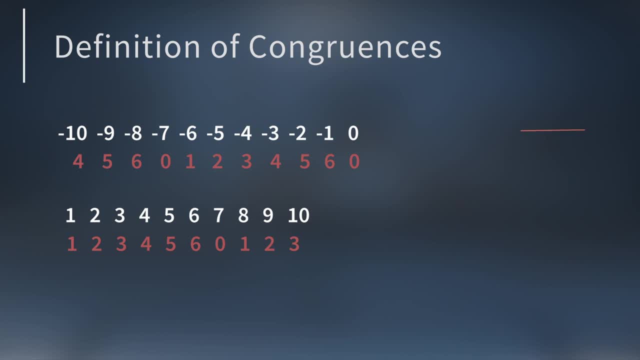 a remainder between 0 and 6.. Even when you divide a negative number by seven, you still get a remainder between 0 and 6.. Let's group the integers into sets by their remainder. The first will be all the integers with a remainder of zero when you divide by seven. 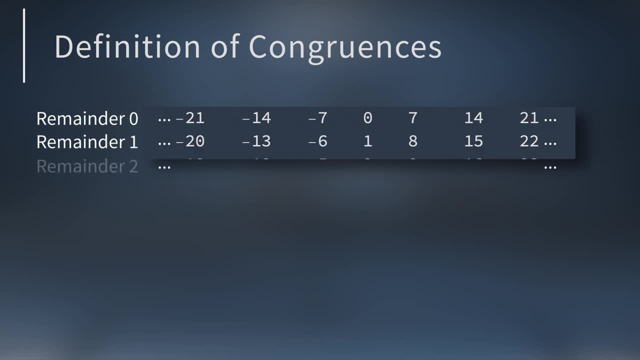 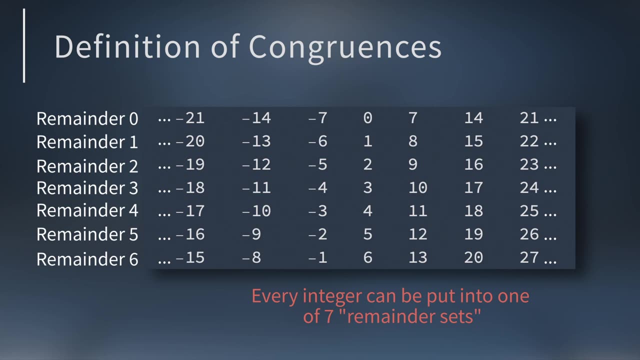 The next will be those with a remainder of one, then two and so on. So every integer can be put into one of seven remainder sets. In each set the integers are seven apart, but the patterns go much, much deeper If you pick any number from one set and add it. 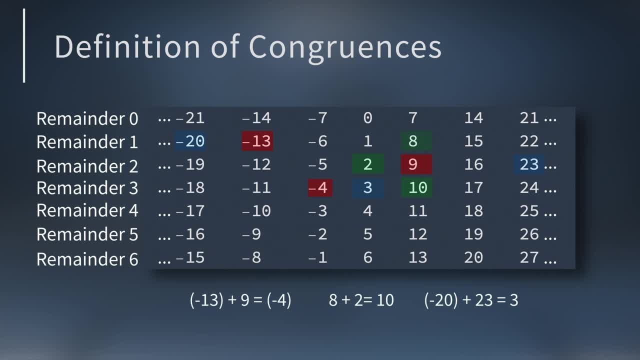 to an integer from another set, then the sum is always in the same set. Try this a few times to feel the excitement yourself. This also works for subtraction and it even works for multiplication. But division, sadly, is different. When you divide one integer, 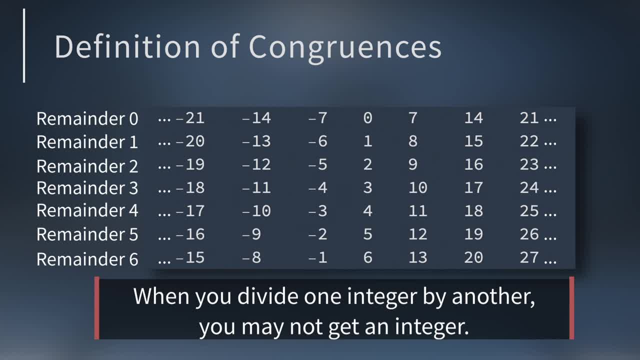 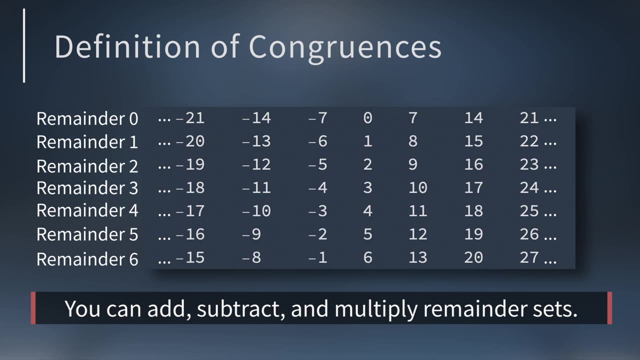 by another, you may not get an integer, So let's set aside division for now and focus on the other three operations. The big idea is this: These remainder sets can be treated as standalone mathematical objects that you can add, subtract and multiply, And we can study these objects and look for. 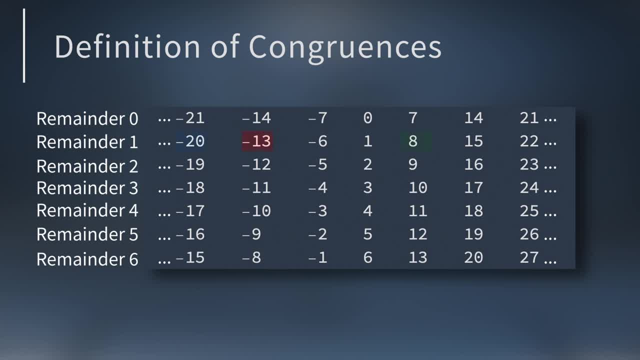 but the patterns go much, much deeper. If you pick any number from one set and add it to an integer from another set, then the sum is always in the same set. Try this a few times to feel the excitement yourself. This also works for subtraction and it even works. 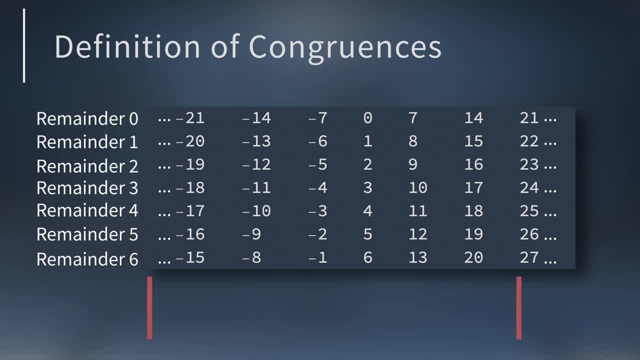 for multiplication. But division, sadly, is different. When you divide one integer by another, you may not get an integer. So let's set aside division for now and focus on the other three operations. The big idea is this: These remainder sets can be treated as standalone mathematical. 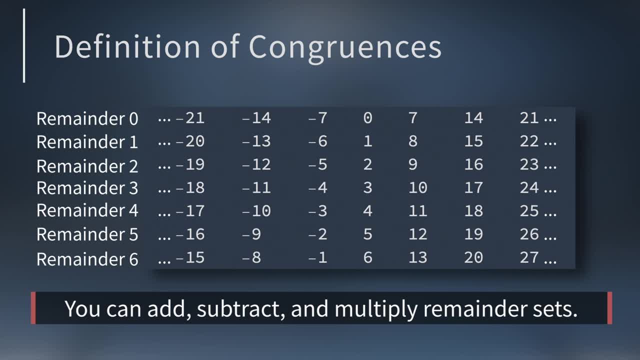 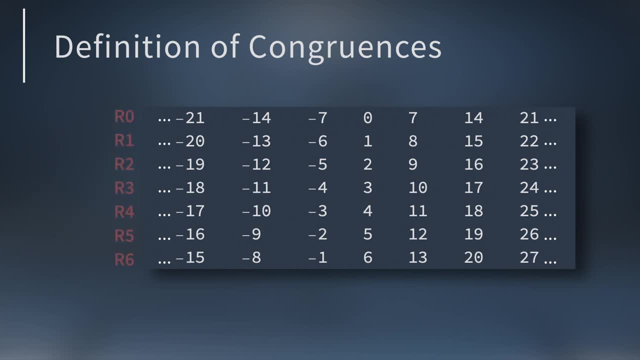 objects that you can add, subtract and multiply And we can study these objects and look for interesting patterns and properties. Let's give each of these seven sets a name. When you add any number with a remainder of three divided by seven to any number from the 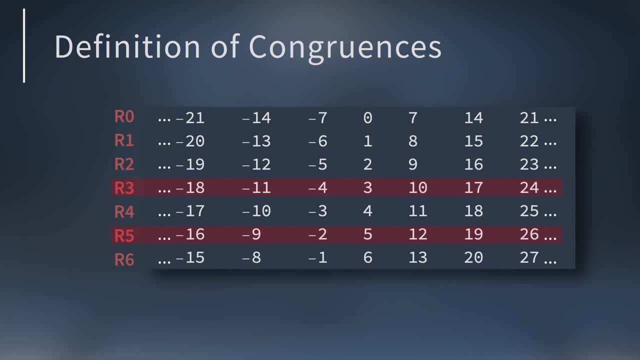 remainder five set. you always get an integer in the remainder one set. We could write this as: r3 plus r5 equals r1.. And, as we saw earlier, you can write down similar expressions for subtraction and multiplication. For example, r2 minus r4 equals r5, and r3 times r3 equals. 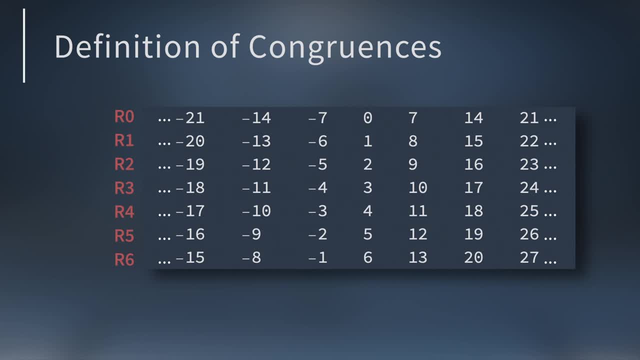 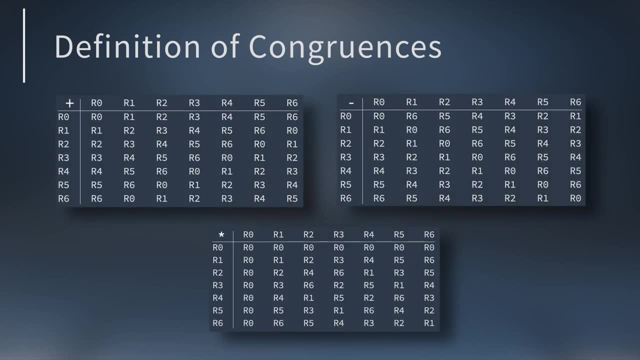 r2.. It's almost as if we've created a new way to do arithmetic- Remainder arithmetic. Here are the addition, subtraction and multiplication tables for these seven remainder sets. Don't forget that we had to put aside division for the time being In mathematics, when you do. 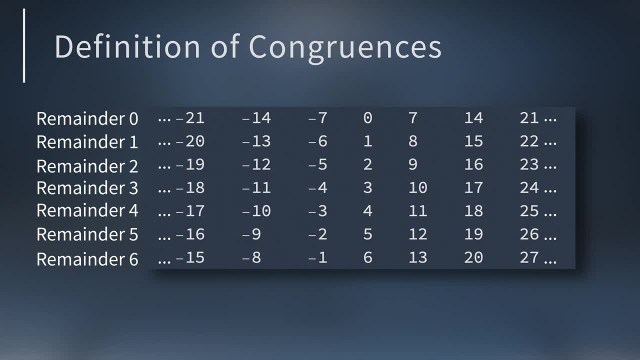 interesting patterns and properties. Let's give each of these seven sets a name. When you add any number with a remainder of three divided by seven to any number from the remainder five set, you always get an integer in the remainder one set. We could write this: 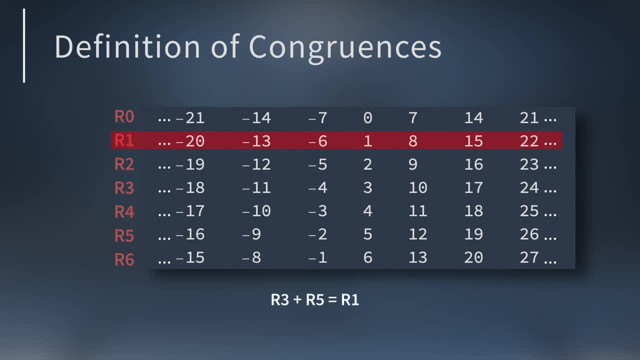 as r3 plus r5 equals r1.. And, as we saw earlier, you can write down similar expressions for subtraction and multiplication. For example, r2 minus r4 equals r5, and r3 times r3 equals r2.. It's almost as if we've created a new way to do arithmetic- Remainder arithmetic- Here. 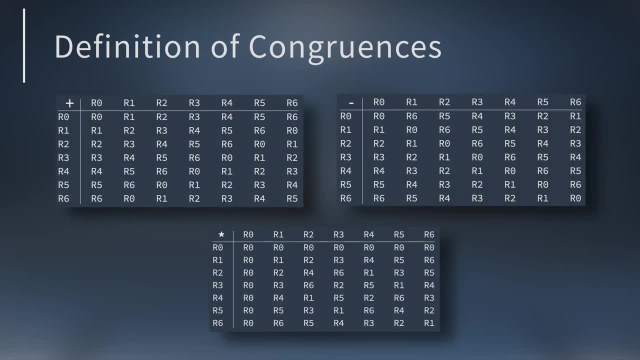 are the addition, subtraction and multiplication tables for these seven remainder sets. Don't forget that we had to put aside division for the time being. In mathematics, when you do arithmetic with the remainder sets, we call it modular arithmetic. There is also some 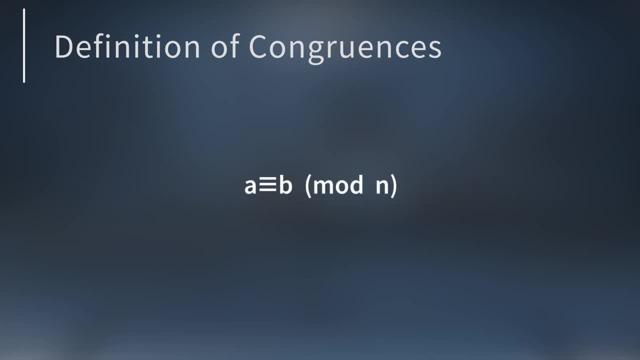 notation that is used when talking about modular arithmetic. What this notation says is that a and b are in the same remainder set when you divide by n. This expression is called a congruence. If two numbers, a and b, are in the same remainder set when you divide by seven, we write it. 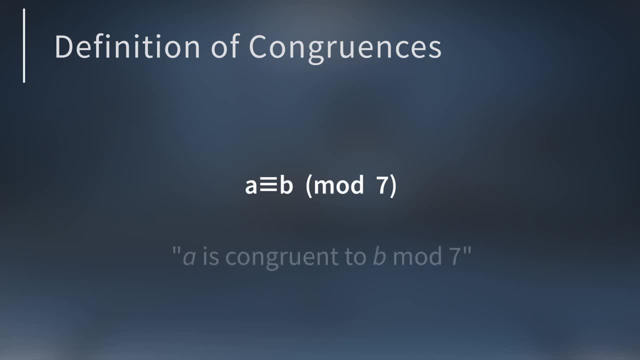 like this. You read this aloud: as: a is congruent to b mod seven. This is the mathematical way to say that a and b have the same remainder when you divide by seven. The symbol with three lines is called the congruence symbol. The number inside parentheses is called the. 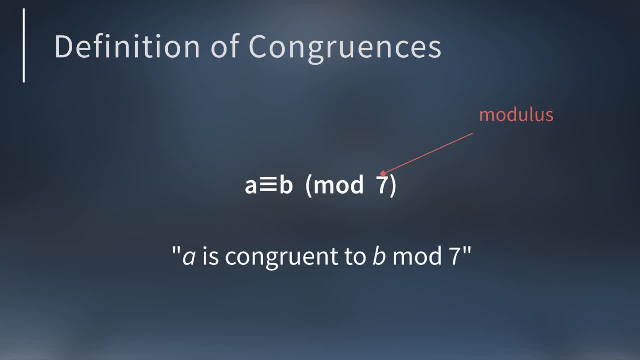 modulus. That's why we write mod inside parentheses. it's short for modulus. So here the modulus is 7.. So far we've focused on the number 7 as a way to motivate the idea of congruences, but now it's time to talk about congruences and modular arithmetic in a more general sense. 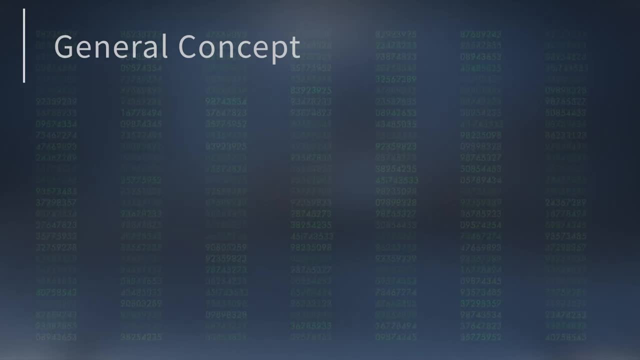 Let's take all of the integers and look at the remainders. when you divide by a positive integer, n, Each integer will have a remainder between 0 and n-1. when you divide by n, We can partition the whole numbers into n sets. based on the remainders Above, we call these: 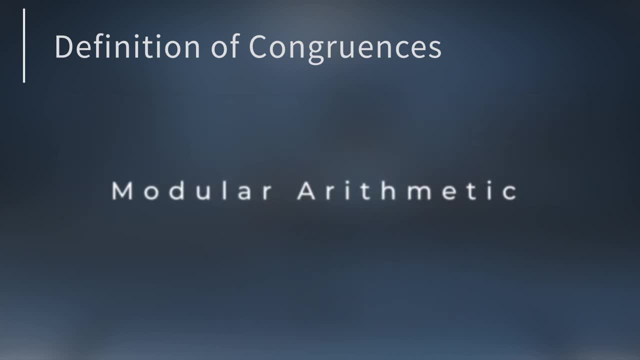 arithmetic with remainder sets. we call it modular arithmetic. There's also some notation that is used when talking about modular arithmetic. What this notation says is that a and b are in the same remainder set when you divide by n. This expression is called a congruence. 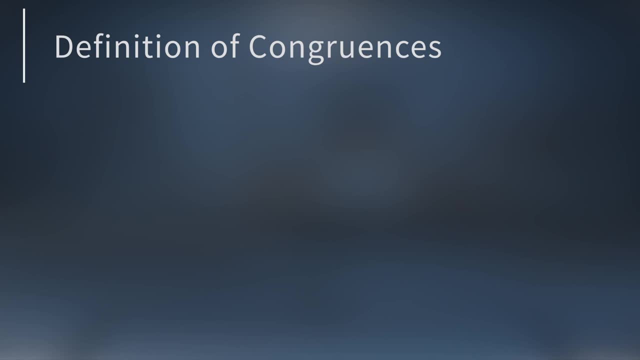 If two numbers, a and b, are in the same remainder set when you divide by seven. we write it like this- You read this aloud: as: a is congruent to b mod seven. This is the mathematical way to say that a and b have the same remainder when you divide by seven. The symbol with: 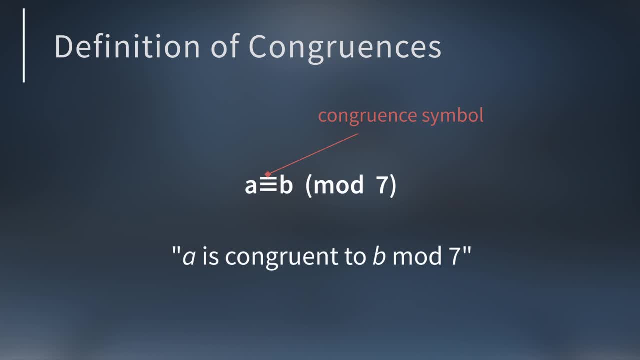 three lines is called the congruence symbol. The number inside parentheses is called the modulus. That's why if we write mod inside parentheses it's short for modulus. So here the modulus is seven. So far we've focused on the number seven as a way to motivate the idea of congruences. 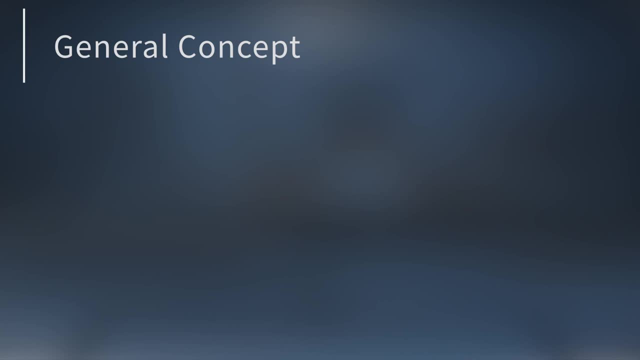 but now it's time to talk about congruences and modular arithmetic in a more general sense. Let's take all of the integers and look at the remainders. when you divide by a positive integer n, Each integer will have a remainder. Let's take r3.. 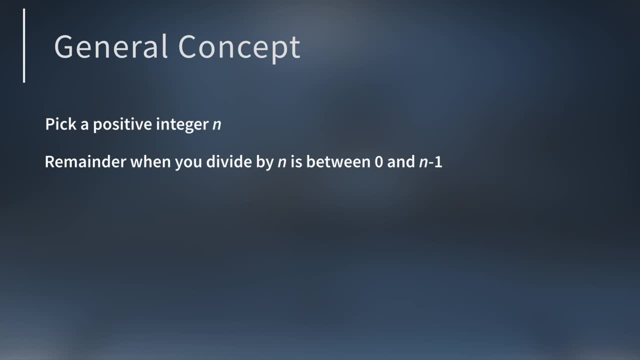 So here you have a positive integer, a nasty integer and a opposite integer on the吃 non VI. So on the top there are three things to activate numbers for this number. One is to generate 0, and n minus 1. when you divide by n, We can partition the whole numbers into n sets. 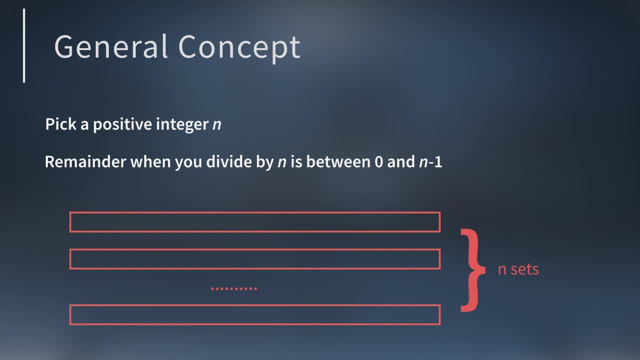 based on their remainders. Above we call these remainder sets, but in number theory you call them congruence classes. Like before, you can add, subtract and multiply two numbers from congruence classes and the result will always be in the same class, So the following: 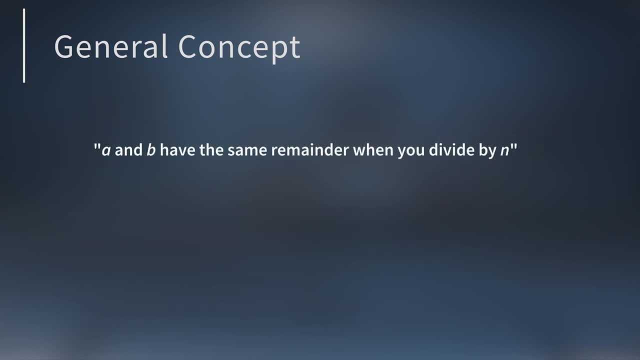 statements mean the same thing. a and b have the same remainder. when you divide by n, a and b are in the same congruence. class a is congruent to b, mod n. These terms and notation will eventually become second nature to you. it's now time to see some examples. 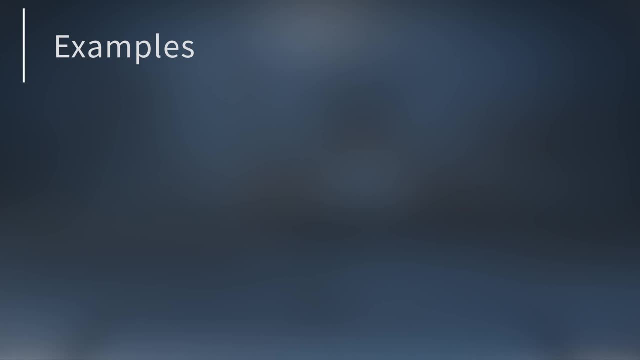 Let's look at some congruences and determine if they are true or false. Is 30 congruent to 12 mod 9? Yes, when you divide 30 by 9, you get a remainder of 3. And the same goes. 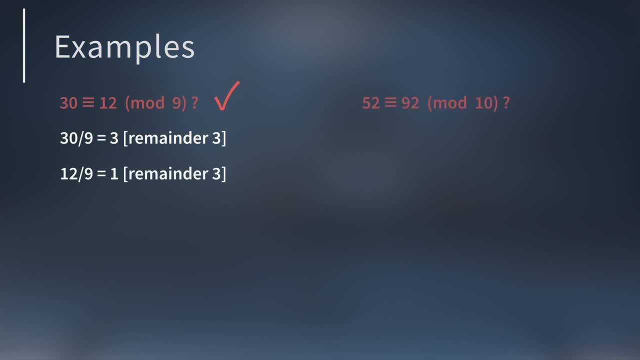 for 12.. Yes, when you divide either number by 10, the remainder is 2.. And what about this congruence? 35 is congruent to negative 1 mod 6.. This is also true: If you divide 35 by 6, you get a remainder of 5.. 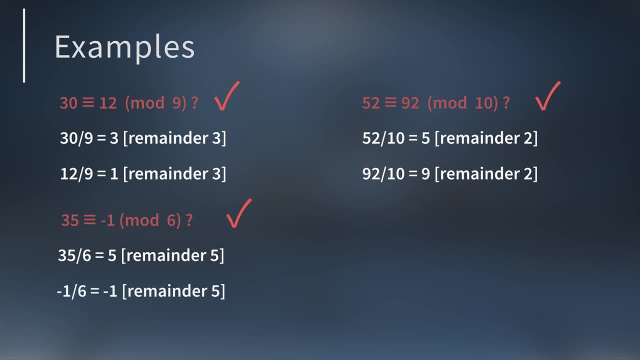 And if you divide negative 1 by 6, you get a quotient of negative 1 and also a remainder of 5.. Is A congruent to A mod 16?? This is also true Even though we don't know the value of A, since both sides of the congruence are the 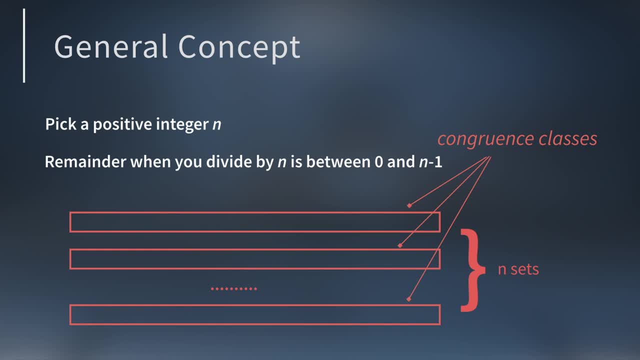 remainder sets, but in number theory you call them congruence classes. Like before, you can add, subtract and multiply two numbers from congruence classes and the result will always be in the same class. So the following statements mean the same thing. 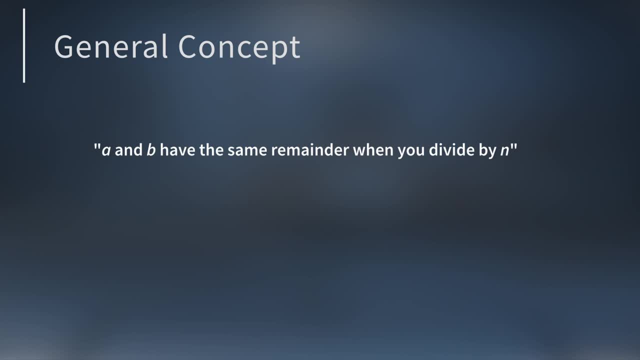 a and b have the same remainder when you divide by n. a and b are in the same congruence. class a is congruent to b mod n. These terms and notation will eventually become second nature to you. It's now time to see. 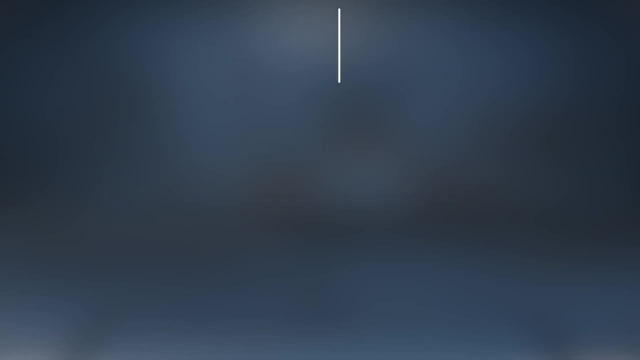 some examples. Let's look at some congruences and determine if they're true or false. Is 30 congruent to 12 mod 9? Yes, When you divide 30 by 9,, you get a remainder of 3, and the same goes for 12.. 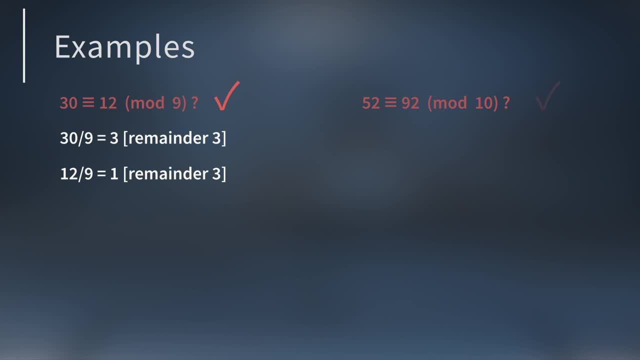 Is 52 congruent to 92 mod 10? Yes, When you divide either number by 10, the remainder is 2.. And what about this congruence? 35 is congruent to negative 1 mod 6.. This is also true If 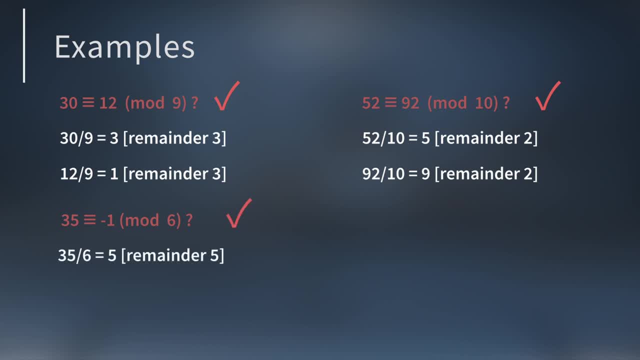 you divide 35 by 6, you get a remainder of 5.. And if you divide negative 1 by 6, you get a quotient of negative 1 and also a remainder of 5.. is A congruent to A mod 16?? This is also true even though we don't know the value of A. 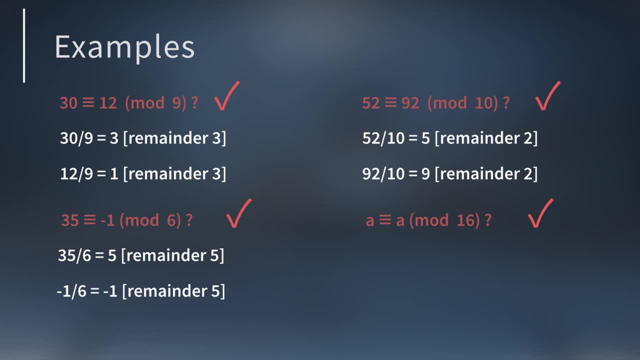 since both sides of the congruence are the same, they'll have the same remainder. How about this? congruence 14 is congruent to 6 mod 5.. This is false. Dividing both numbers by 5,, 14 has a remainder of 4, and 6 has a remainder of 1.. So these two are not congruent mod 5.. 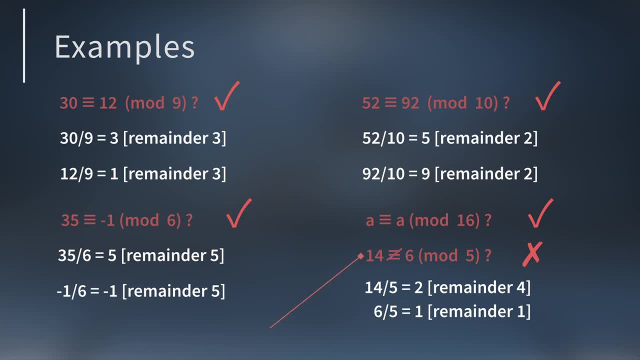 When the congruence is not true, you draw a slash through the congruence symbol. There's a useful trick to check if two numbers are congruent. Above we did several divisions to see if each congruence was correct or not. We divided both sides by the modulus and checked if. 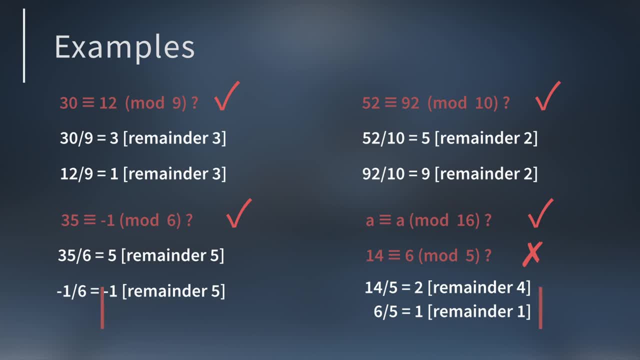 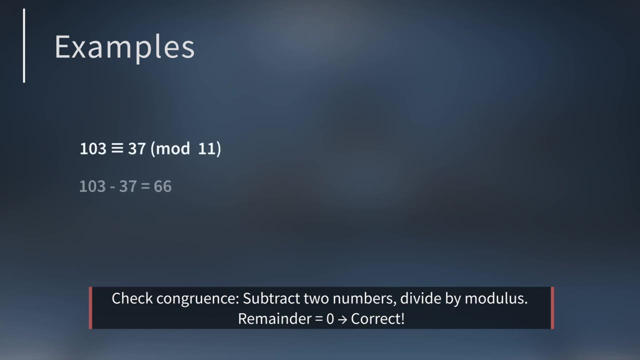 the remainders were the same. Another way you can check is by subtracting the two numbers. the order doesn't matter. then divide by the modulus. If the remainder is 0, then the congruence is correct. For example, is 103 congruent to 37 mod 11?? If you subtract the two numbers, you get 66.. 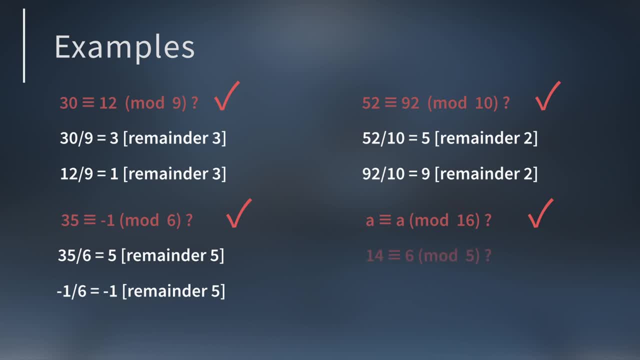 same. they'll have the same remainder. How about this congruence? 14 is congruent to 6 mod 5.. This is false. Dividing both numbers by 5, 14 has a remainder of 4 and 6 has a remainder of 1.. 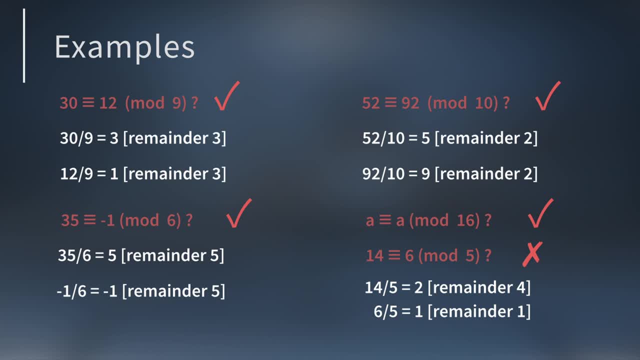 So these two are not congruent, mod 5. When the congruence is not true, you draw a slash through the congruence symbol. OK, There's a useful trick to check if two numbers are congruent. Above we did several divisions to see if each congruence was correct or not. 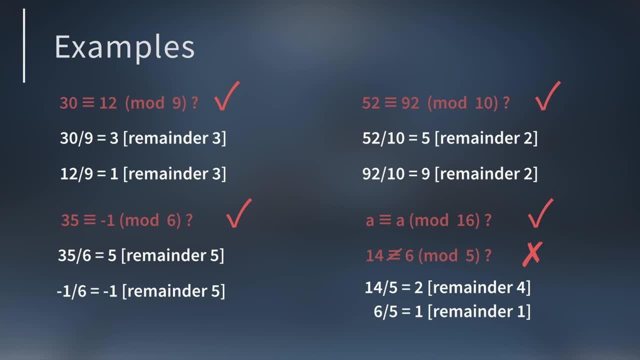 We divided both sides by the modulus and checked if the remainders were the same. Another way you can check is by subtracting the two numbers- the order doesn't matter- then divide by the modulus. If the remainder is 0,, then the congruence is correct. 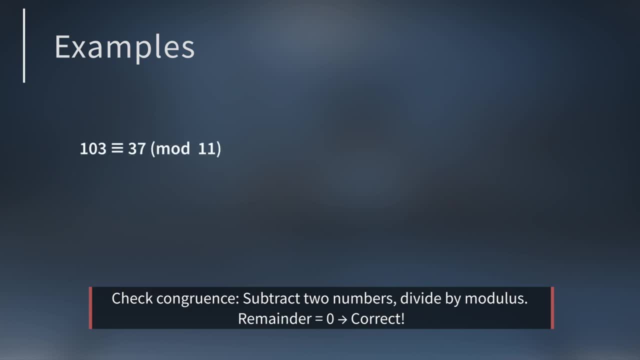 For example, is 103 congruent to 37 mod 11?? If you subtract the two numbers, you get 7.. If you subtract the two numbers, you get 66.. When you divide 66 by the modulus 11,, you get a remainder of 0. 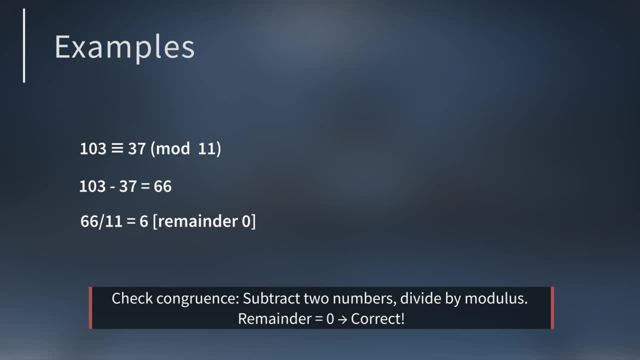 In other words, 66 is a multiple of 11, so this is correct. To see why this trick works, look at the general case. a is congruent to b mod n. If this is true, then dividing a and b by n will give you the same remainder r. 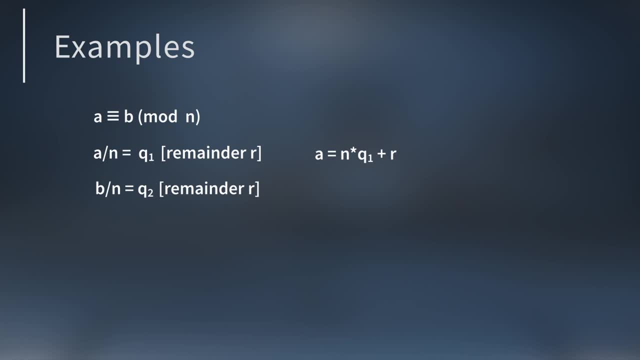 So a equals n times q1 plus r And b equals n times q2 plus r, Where the q's are the quotients. If you subtract these two expressions, you get a minus b equals n times the quantity of q1 minus q2.. 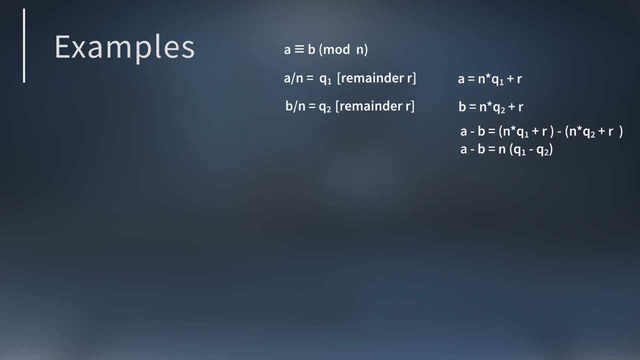 So a minus b is a multiple of n. We've shown that if a is congruent to b mod n, then it's true that n divides a minus b. However, it's also important to flip this statement and show the reverse is true. 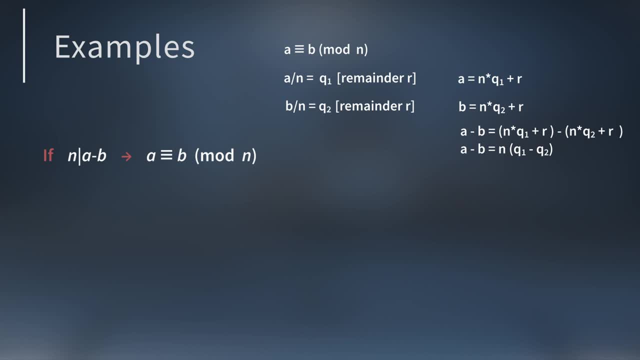 That is, if n divides a minus b, then a is congruent to b mod n. So we've shown that if n divides a minus b, then a is congruent to b mod n. So we've shown that if n divides a minus b, then a is congruent to b mod n. 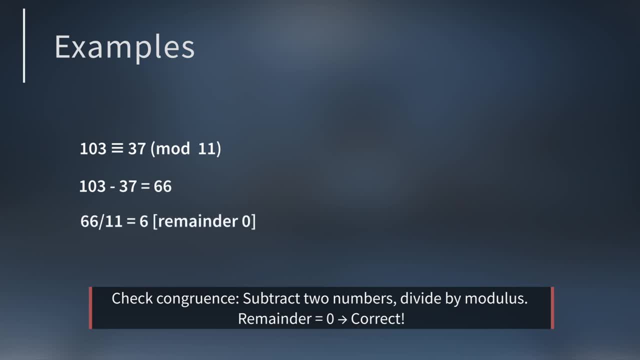 When you divide 66 by the modulus 11, you get a remainder of 0. In other words, 66 is a multiple of 11, so this is correct. To see why this trick works, look at the general case. A is congruent to B mod N. If this is true, then dividing A and B by N will give you the. 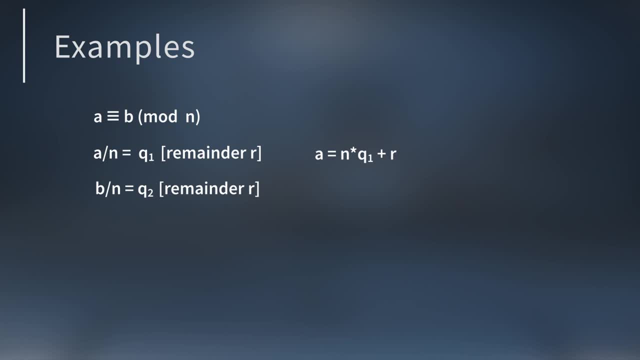 same remainder R. So A equals N times Q1 plus R and B equals N times Q2 plus R, where the Qs are the quotients. If you subtract these two expressions, you get A minus B equals N times the quantity of Q1 minus. 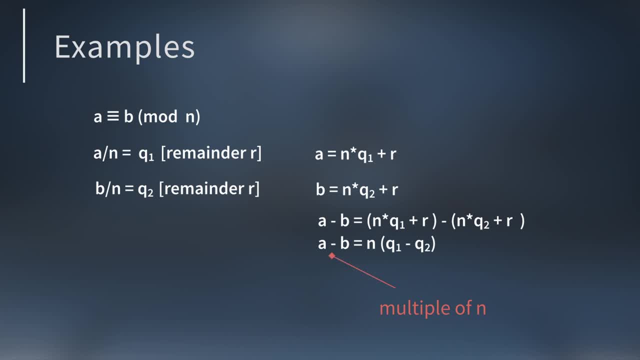 Q2.. So A minus B is a multiple of N. We've shown that if A is congruent to B mod N, then it's true that N divides A minus B. However, it's also important to flip this statement and see if the reverse is true, That is, if N divides A minus B, then A is congruent to B mod N. 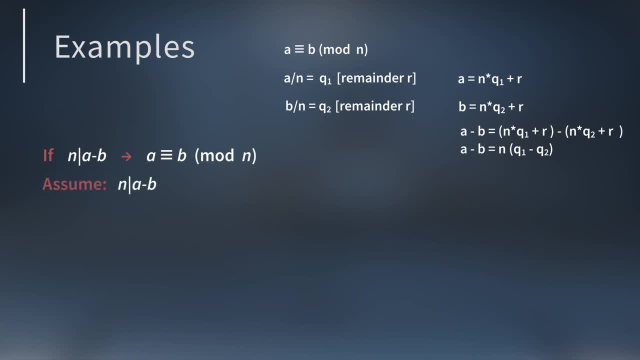 To see this, let's assume that N divides A minus B. Next, suppose that when you divide A by N, the remainder is R1, and when you divide B by N, the remainder is R2.. This means A equals N times Q1 plus R1, and B equals N times Q2 plus R2.. 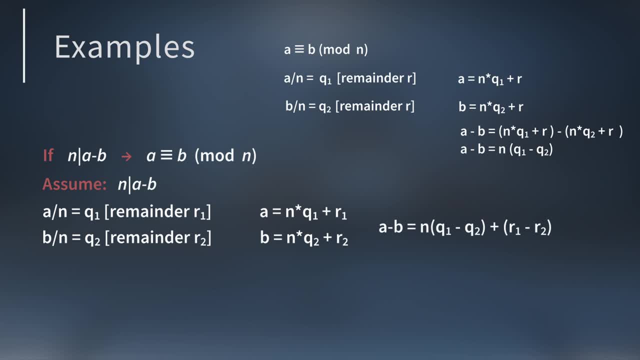 So A minus B equals N times the quantity of Q1 minus Q2, plus the quantity of R1 minus R2.. If N divides A minus B on the left, then N divides the right hand side too. N divides the first term, since it's a multiple of N. This means that N has to divide R1 minus R2.. 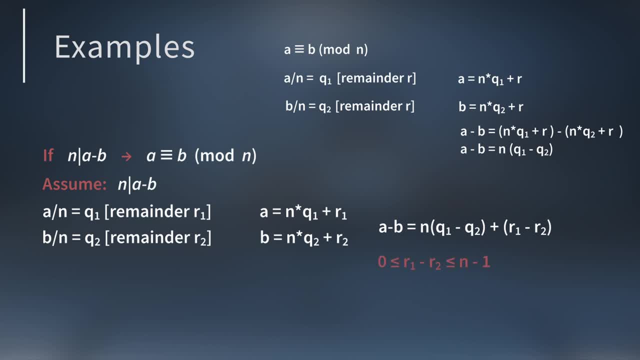 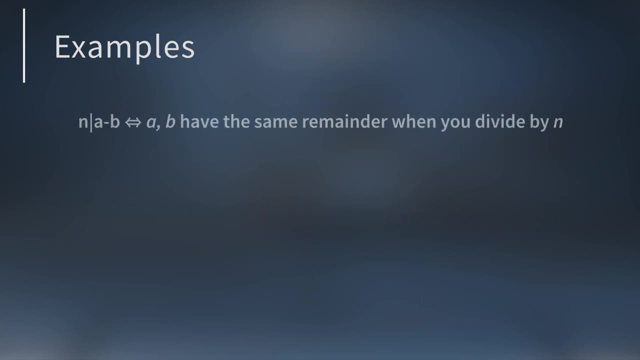 But since the remainders are both between 0 and N minus 1, the only way N can divide this evenly is the remainder, as кус there is 0. This is then R1 equals R2, theheld Well A is congruent to B mod N, Since N divides A. 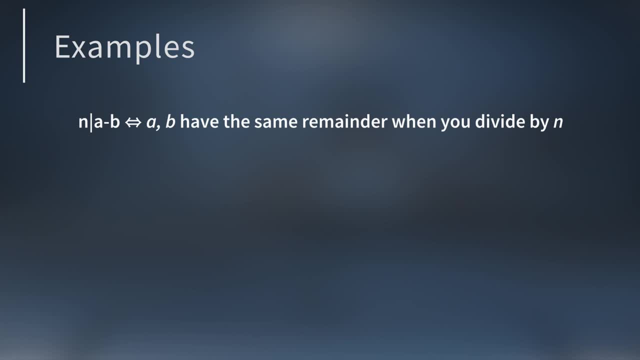 minus B means A and B have the same remainder when you divide by N. some people will define A is congruent to B mod N as saying A and B have the same remainder when you divide by N, while others will define it to mean N divides A minus B. 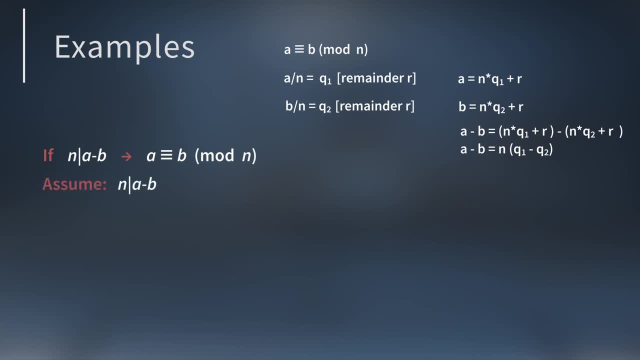 To see this, let's assume that n divides a minus b. Next, suppose that when you divide a by n, the remainder is r1.. And when you divide b by n, the remainder is r2.. This means a equals n times q1 plus r1, and b equals n times q2 plus r2.. 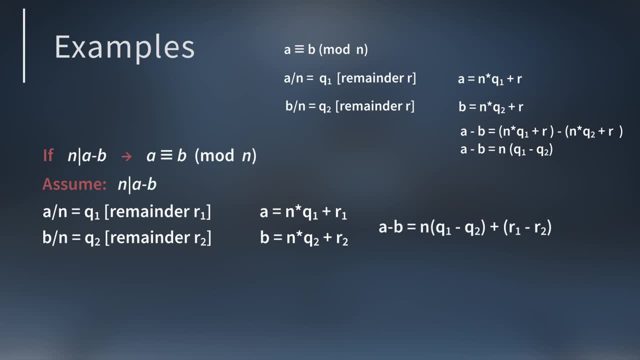 So a minus b equals n times the quantity of q1 minus q2 plus r2.. If n divides a minus b on the left, then n divides the right hand side too. n divides the first term, since it's a multiple of n. 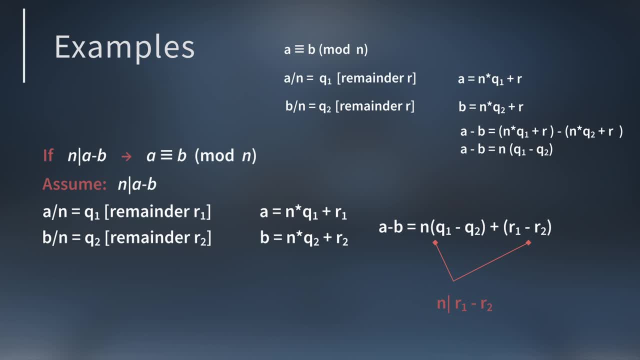 This means that n has to divide r1 minus r2.. But since the remainders are both between 0 and n minus 1, the only way n can divide this evenly is if their difference is 0. This means r1 equals r2.. 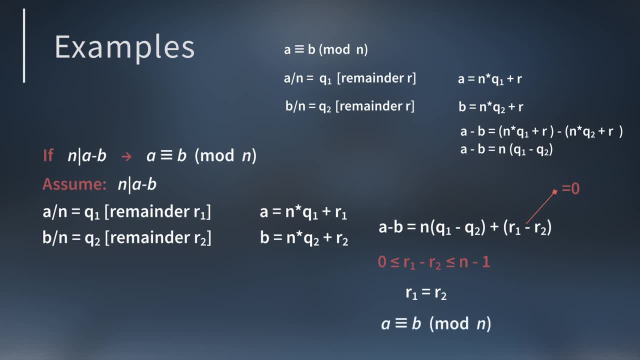 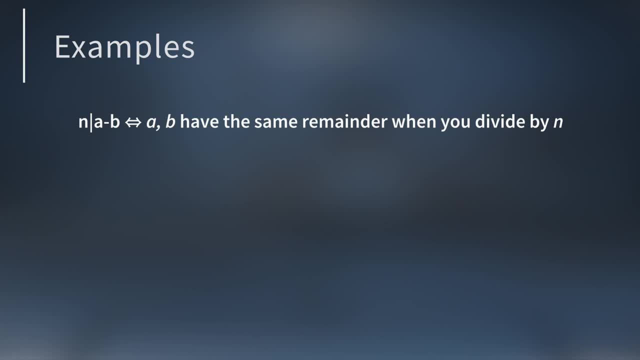 The remainders are the same. So a is congruent to b mod n. Since n divides a minus b means that a and b have the same remainder. when you divide by n and vice versa, some people will define a is congruent to b mod n as saying a and. 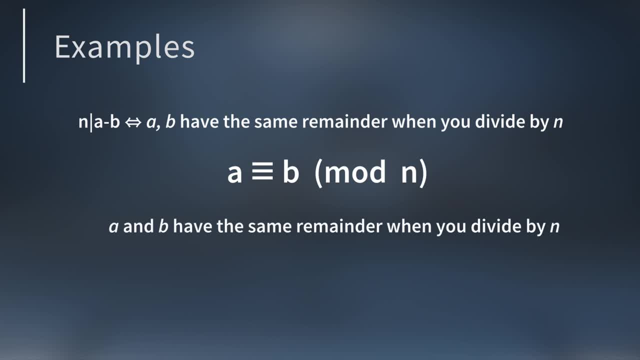 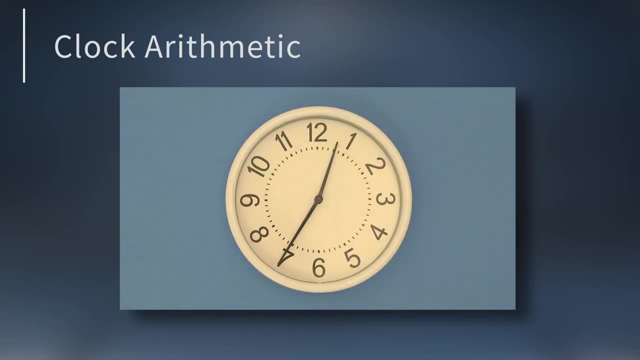 b have the same remainder when you divide by n, while others will define it to mean n divides a minus b. Both definitions are fine. They mean the same thing: 1. 1. 1. 1. 1. 1.. 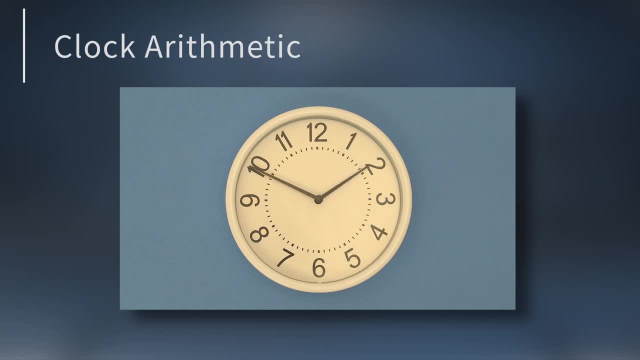 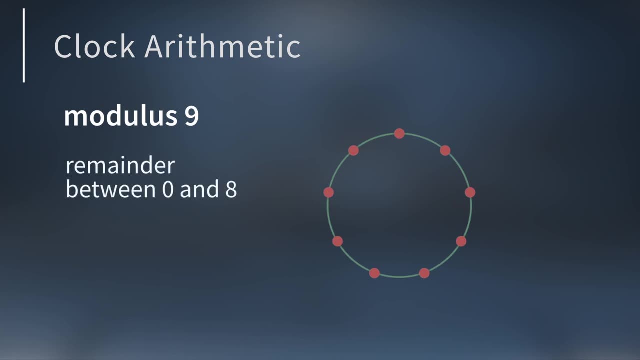 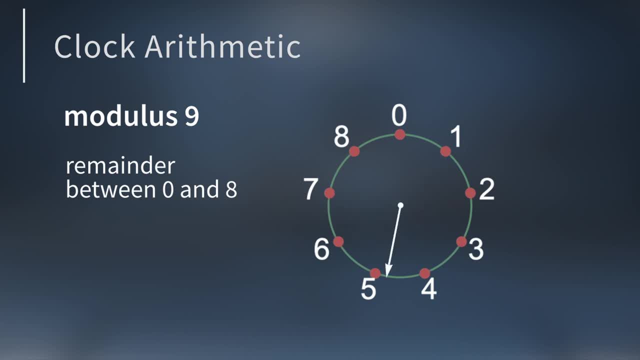 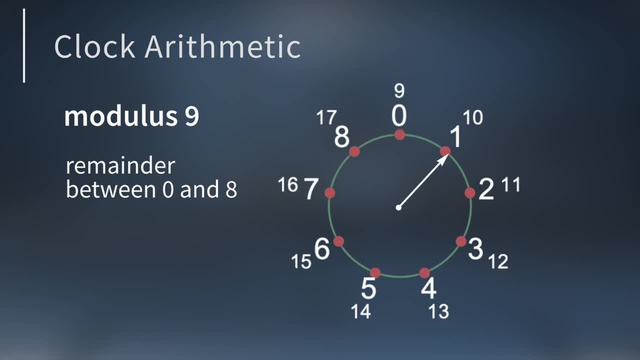 each number next to the corresponding remainder. With this technique, each positive integer appears next to its remainder. So each sector of the clock contains the numbers in each congruence class, And if we start at 0 and count down by going counterclockwise, we can.